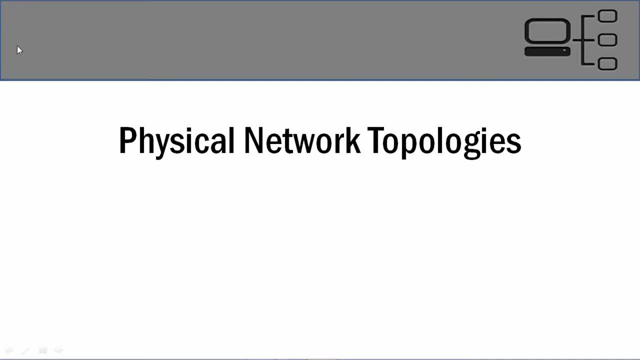 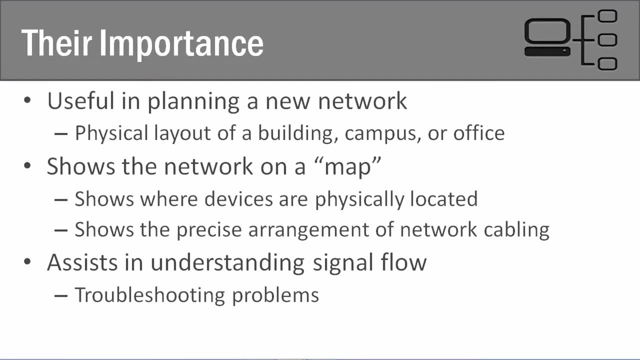 topologies that we're not going to cover in this course. So let's go ahead and let's talk about their importance. So why are physical network topologies important? Well, first of all, it's all about planning, And when we're planning and designing a network, we need to know what type 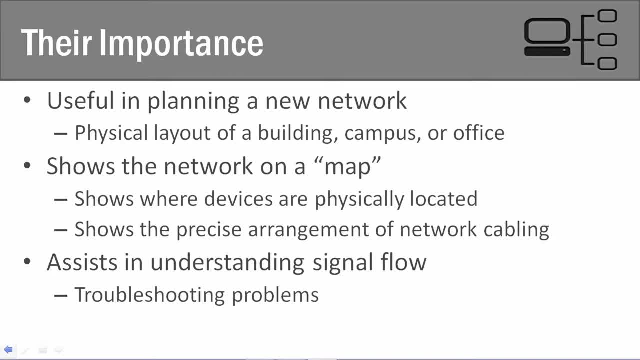 of topology is going to work best for us and for our situation in our network. So we're going to need to know all of our constraints and also, in regards to all of our constraints, Maybe we have technological constraints, or we have monetary constraints, or we even have personnel resource. 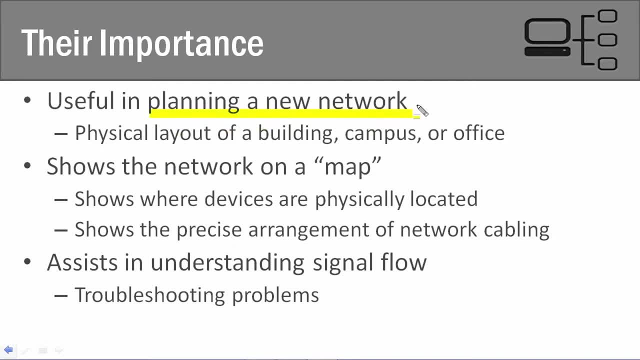 constraints. So it all comes down to planning and designing the network and understanding what's going to work best for you. Another important thing is that it shows the network on a map, And so it's going to physically show where all the devices are on the network, And it's really 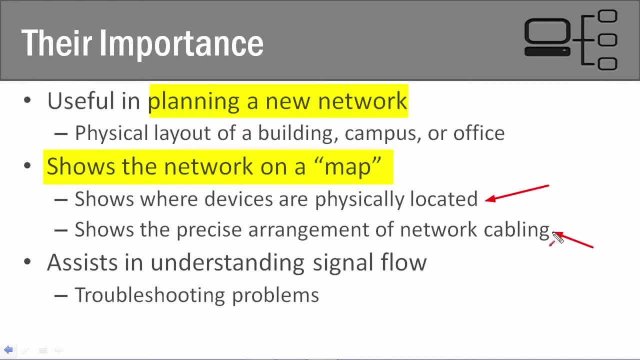 going to show you how everything interacts with the cabling, And for somebody that's been in IT- you've been in desktop support or you've been in network support- you'll know how important this is. And when you don't have this in place, you know how difficult it can make your life, Because 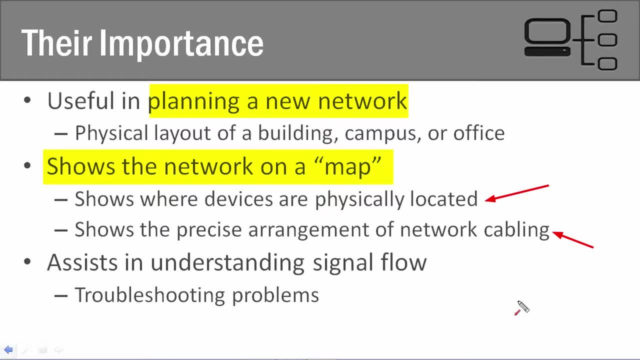 when you don't know how the network's connected and you're having network issues, then not having a physical map in the network is just going to be a huge hindrance for you trying to troubleshoot those issues. So you know when we're talking about all that it really comes down to when you 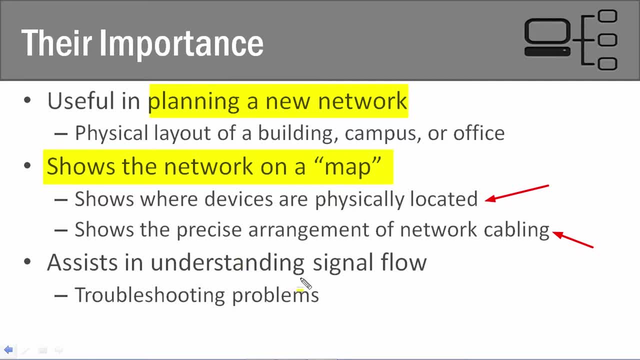 know everything's connected together on a physical map in house design. you understand how data and information flows throughout the network, And so when we're troubleshooting, it's easier to identify what their potential problems are and we can isolate them a lot easier, And so this is what it's all about. This is why it's important We do it, because we need. 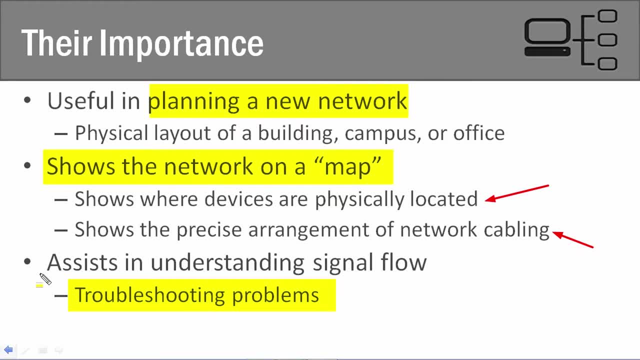 to have network map. Once the network is designed, we need to have one in place for when we design it. we need to understand all our constraints and our resources and understanding how we can properly plan and design the network and what should work for us. And then when we're troubleshooting after. 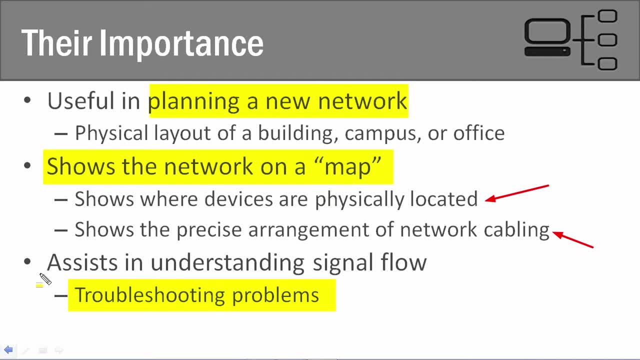 the fact, when we're giving the network off to the system administrators and the network support personnel and the desktop support, it's important for them to have this information so they can easily troubleshoot their issues. So in the next video we're going to start. talking about some of the physical topologies, So I'll see you there.